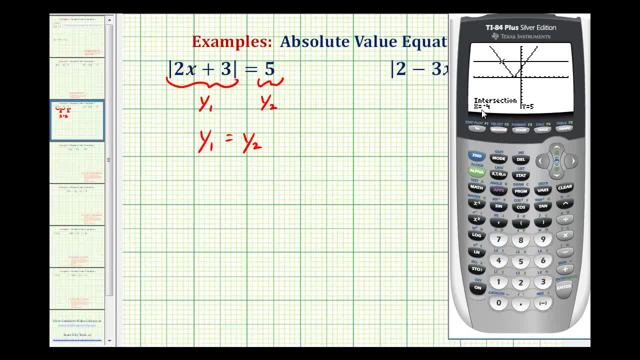 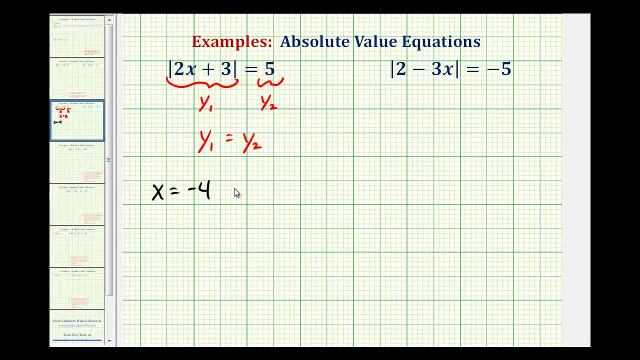 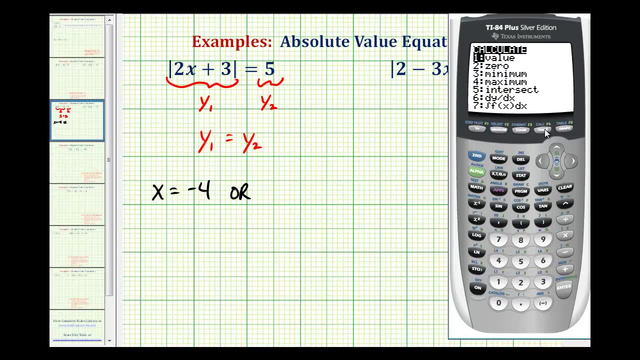 of intersection is: x equals negative 4, which is one of our solutions. We'll go ahead and write that down, And now we'll go back and find the second solution. So we'll do the same thing. We'll press second trace, option 5, move the cursor close to the second point of intersection. 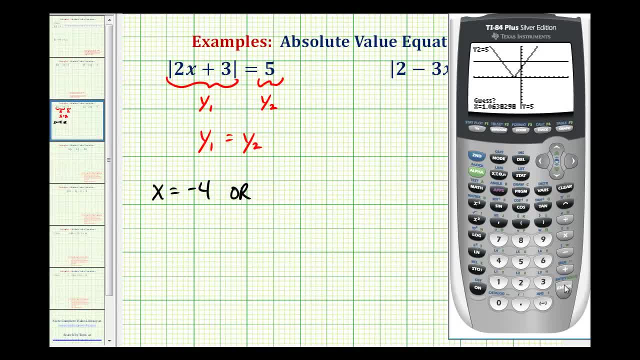 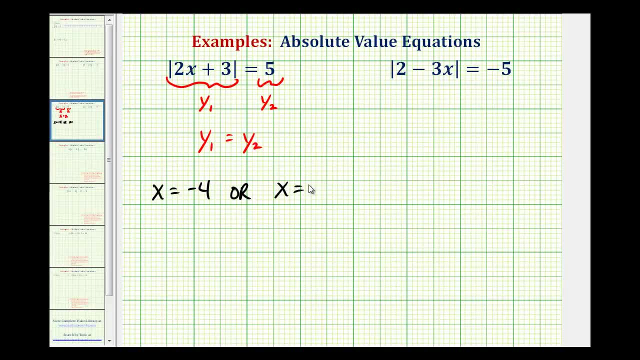 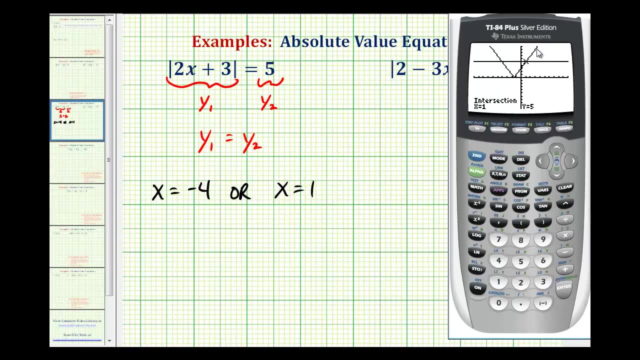 And then enter, enter, enter And now we have x equals 1.. So our solutions are x equals negative 4 or x equals 1.. And hopefully, graphically, you can see now why many absolute value equations have two solutions. If you have a v-shaped graph and a horizontal line, many times they will intersect. 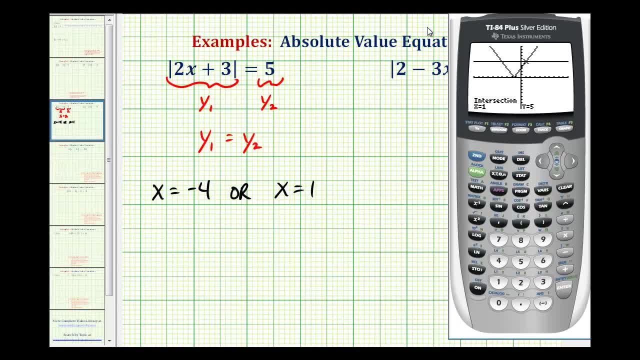 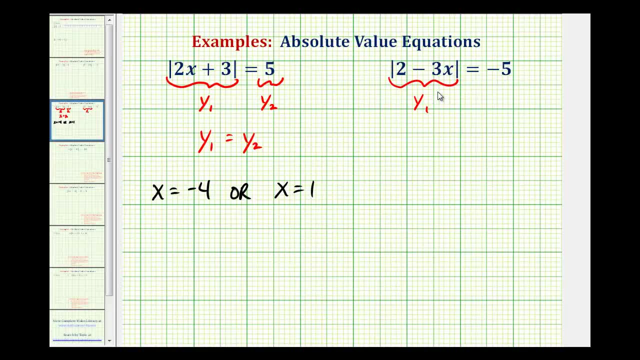 in two points, giving us two solutions. Now let's take a look at the second equation. We're going to do the same thing. We'll let y1 equal the left side and y2 equal the right side, And then we'll see if, graphically, we can determine when these two graphs are equal. 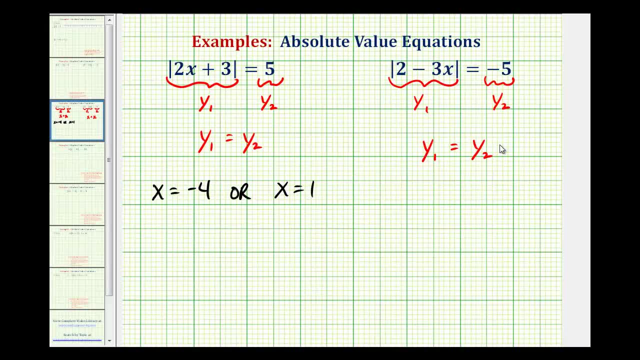 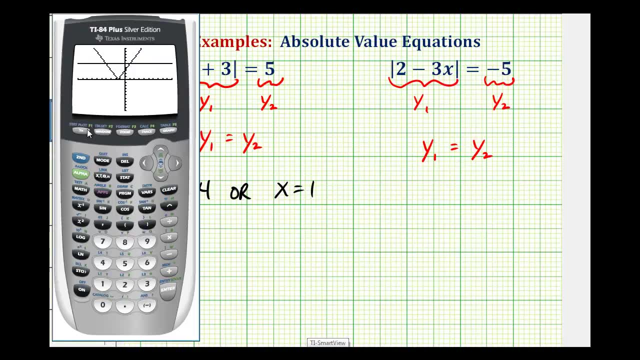 to each other or when they intersect. Now you might notice something special about this equation. Let's go ahead and take a look at the graph. So we'll press y equals. I'm going to go ahead and clear these again And just start from the beginning. 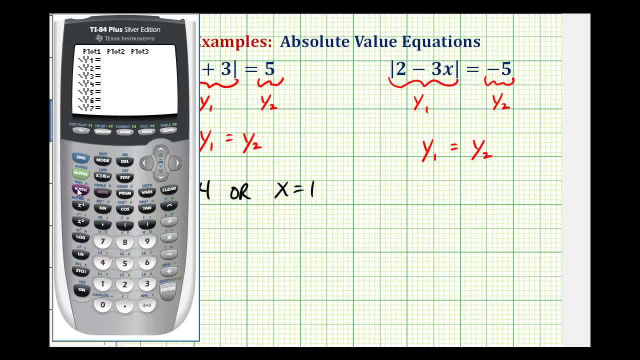 So again we're going to press math right arrow once and then enter for absolute value And then we'll type in 2 minus 3x, close the parenthesis, press enter And then y2 is equal to negative 5.. 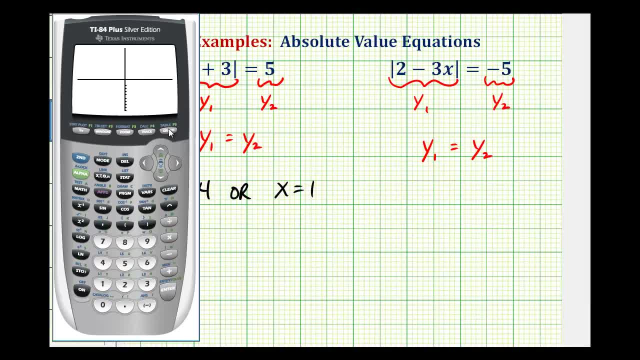 We'll go ahead and press graph And you'll notice there's our v, But notice how the horizontal line is below it. So we're going to press enter. So we're going to press enter. So we're going to press enter. 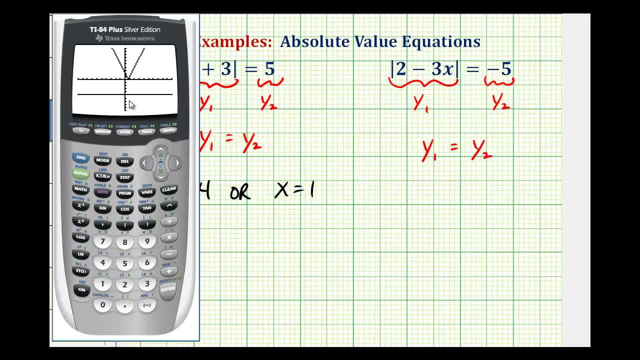 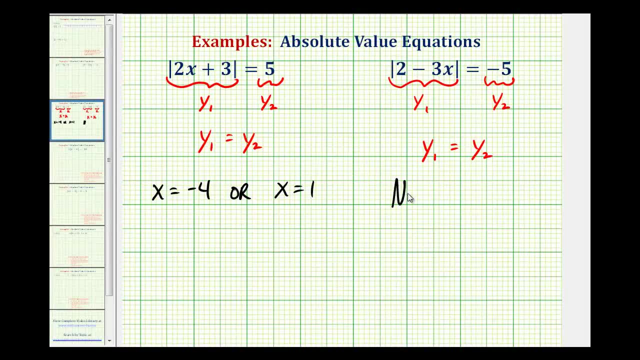 And then we're going to press enter, And then we're going to press enter. This is what it looks like graphically, when there are no solutions to an absolute value equation- And you may have recognized this from the beginning, because we know absolute value is always positive.